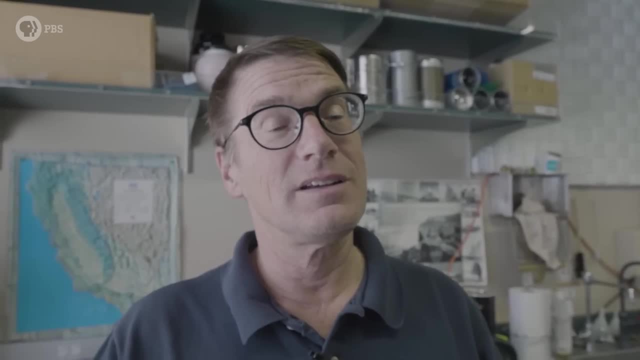 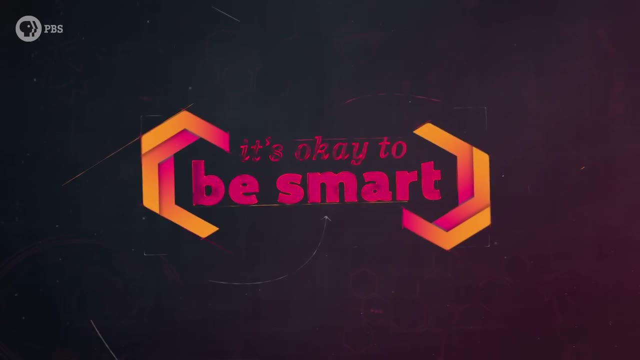 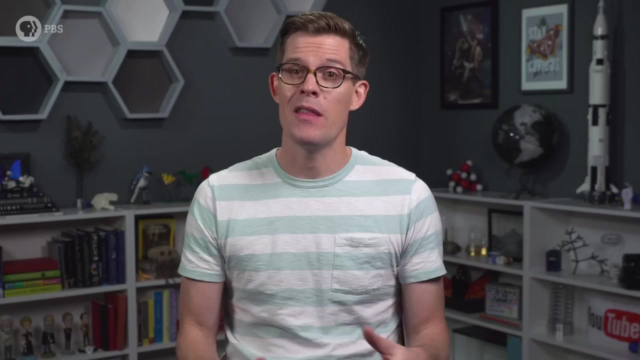 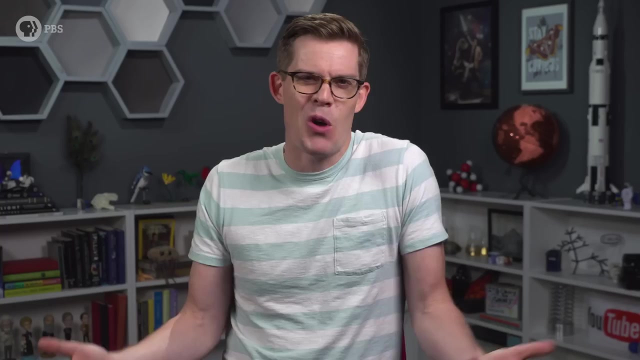 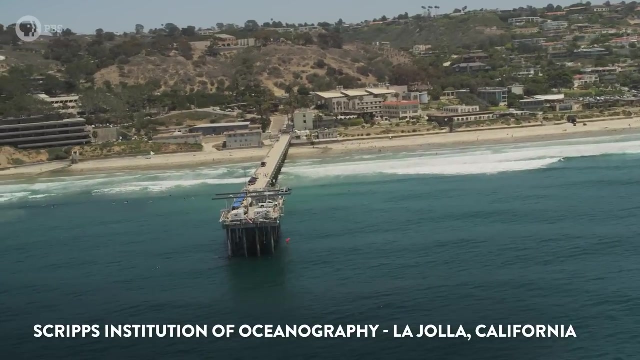 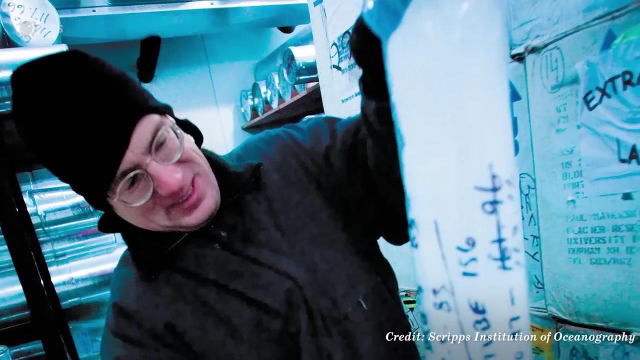 But that's less certain. So it's really quite a dramatic thing that we humans have done to the carbon dioxide. No, because at places like the Scripps Institution of Oceanography in Southern California we have freezers full of ancient ice that let us look into the past thousands, even millions of years and measure exactly what Earth's atmosphere and its climate were like throughout deep history. 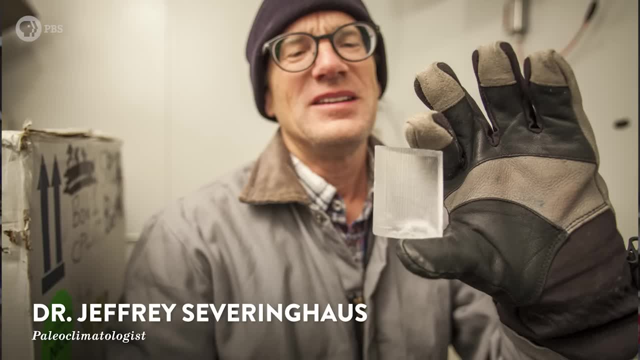 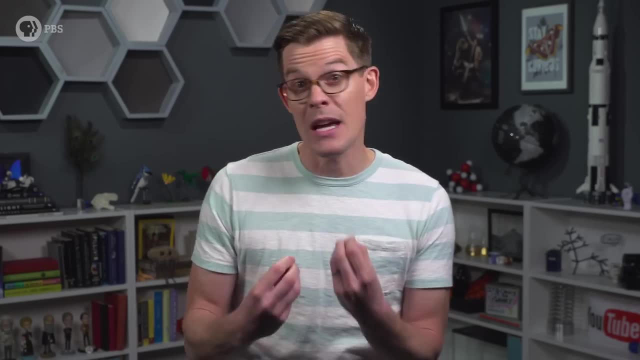 I recently stopped by to visit Dr Jeffrey Severinghouse, who studies ice cores. He's part of a team that's working to find the oldest ice on Earth, Because each of these little blocks of frozen water can tell us something about our planet's past, long before we existed. 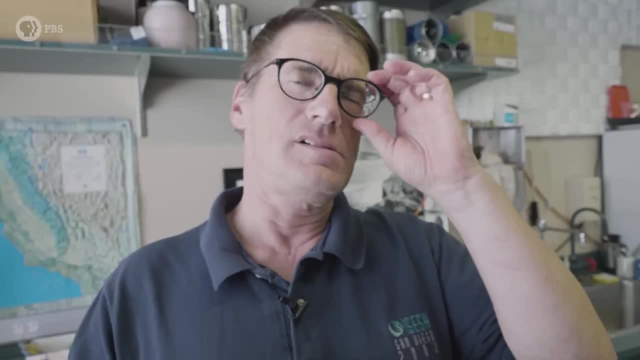 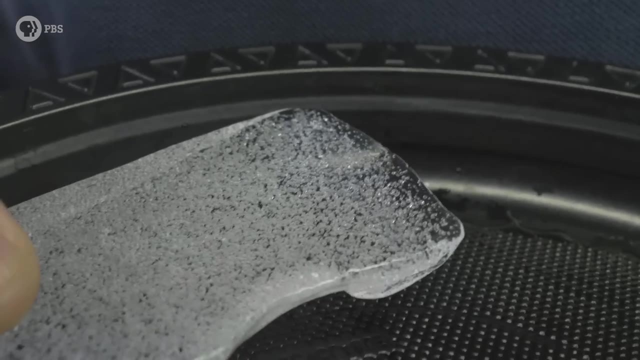 And where it's heading now that we do. And inside these tiny bubbles in this ice are old bubbles of air that existed on this planet as old as that ice is. How's the atmosphere from the planet trapped in those little bubbles? What happens in the polar regions is it's too cold to melt. 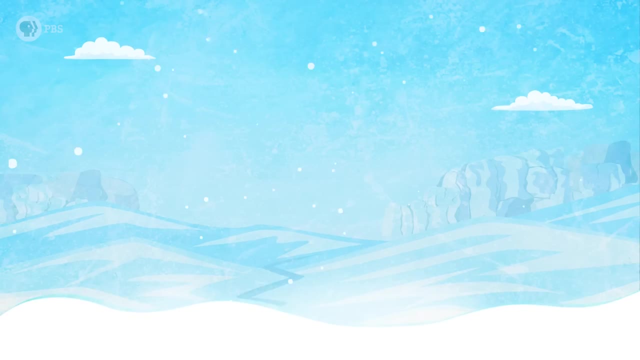 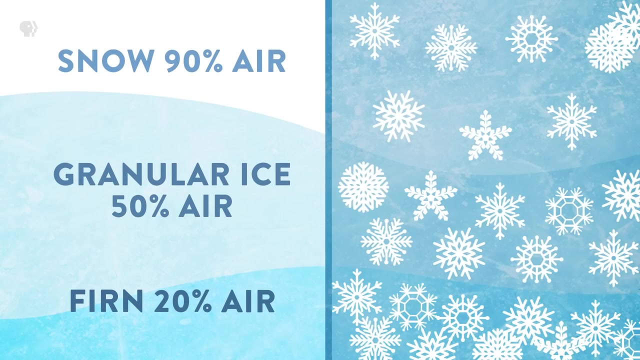 So when snow falls, it doesn't melt, It just piles up and piles up, and piles up and eventually turns into ice, just from under its own weight. You think about what snow is like: You've got a snowflake, but you've got air in between the snowflakes, right? 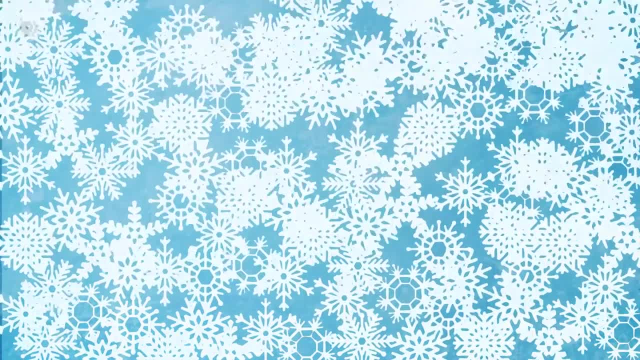 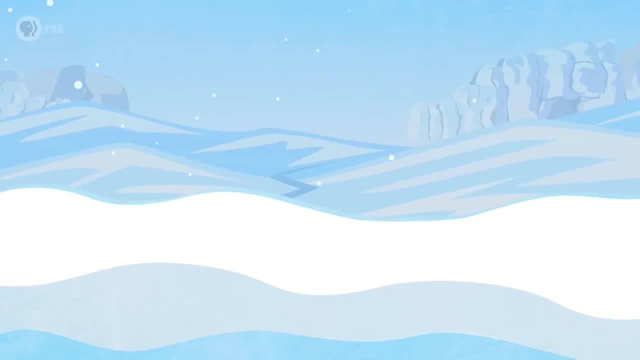 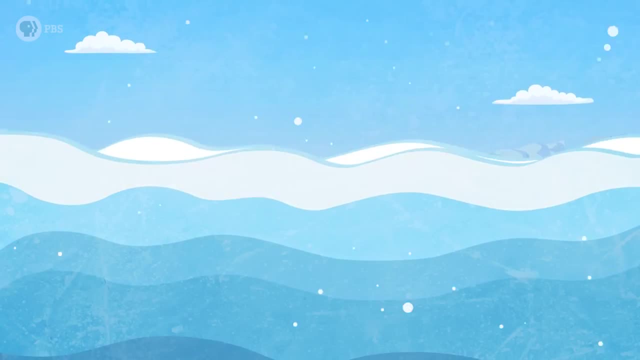 And so, as that snow becomes more and more dense, it tends to squeeze out the air in between the snowflakes, but it turns out it doesn't squeeze out all the air. As more layers of snow fall and condense, those tiny voids are literally frozen in time, layer upon layer, And there are a lot of layers. 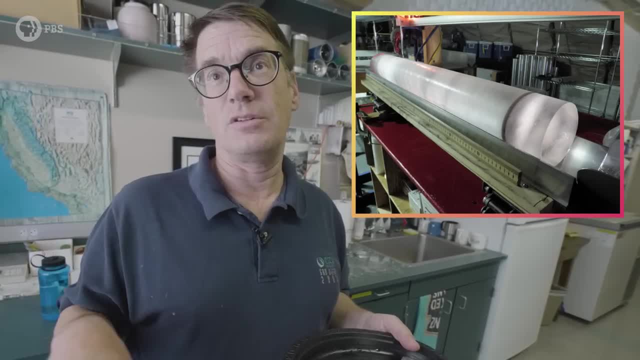 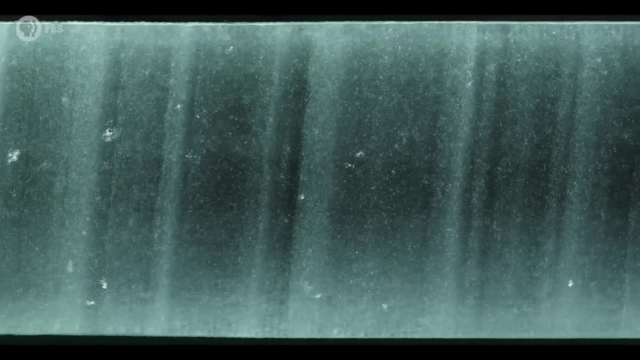 Some ice cores have annual layers, just like trees. do you know, and how you can count tree rings to figure out how old it is? So some graduate student sits there and counts 50,000 annual layers. Of course there has to be a graduate student that's doing that. 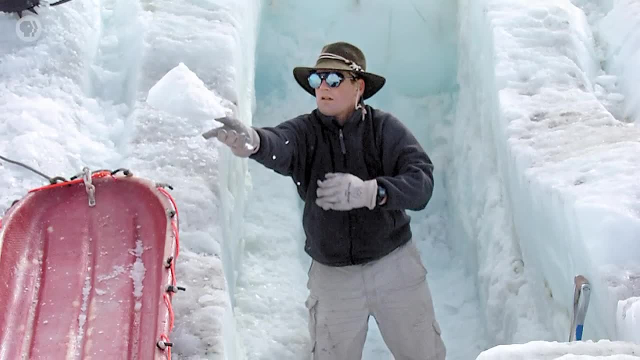 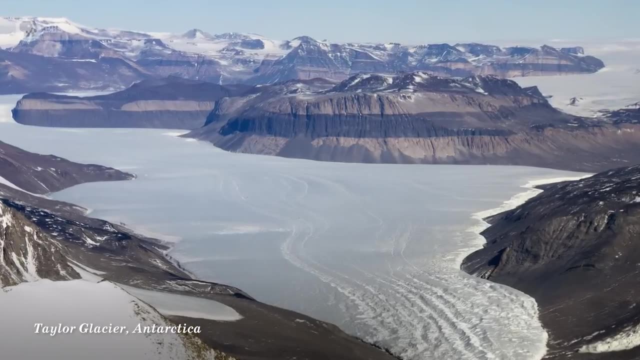 What a lot of work. But to study ancient ice first you have to find ancient ice. Where are you doing this research? Where are you collecting these ice cores? So this is from a place called Taylor Glacier in Antarctica. Taylor Glacier is a 54-kilometer stretch of ice and rock. 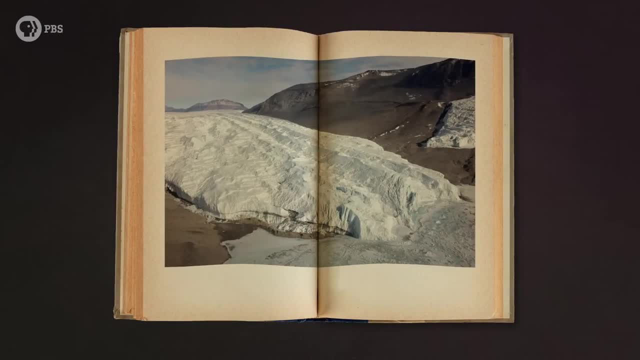 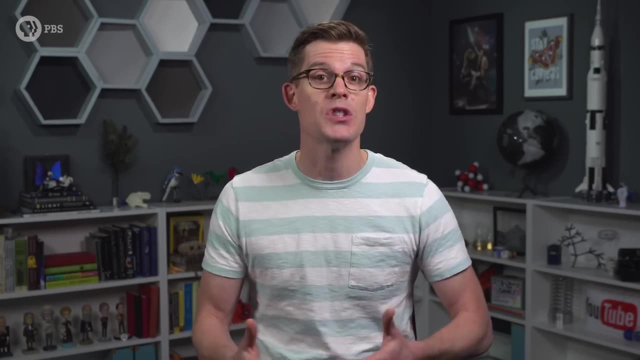 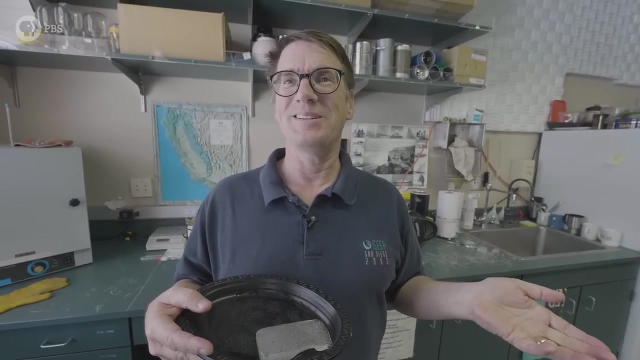 People like Dr Severinghouse can read it like a book full of stories about our ancient climate. Taylor Glacier is a special place because it's one of the few spots on Earth where the ancient ice has risen to the surface, So you only have to drill down, you know, maybe 5,, 10 meters to get the ice. 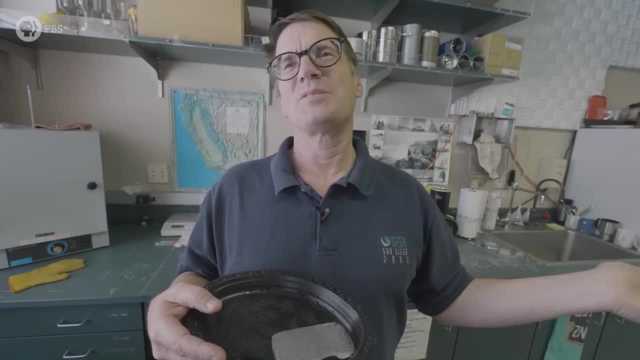 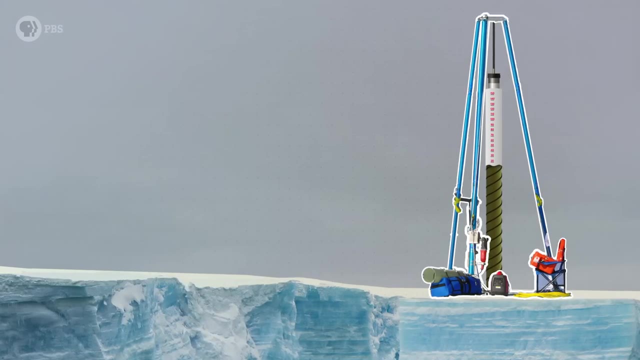 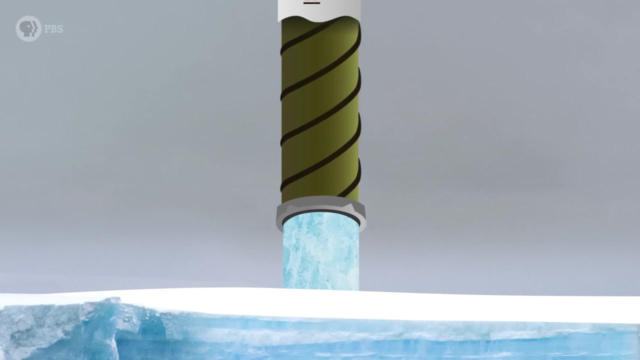 Much easier than drilling a deep ice core, which is, you know, 3,000 meters and costs $50 million. It's basically a cylinder that has tiny little teeth on the bottom And when you rotate the barrel it carves out the ice on the edges and leaves behind an ice core in the middle. 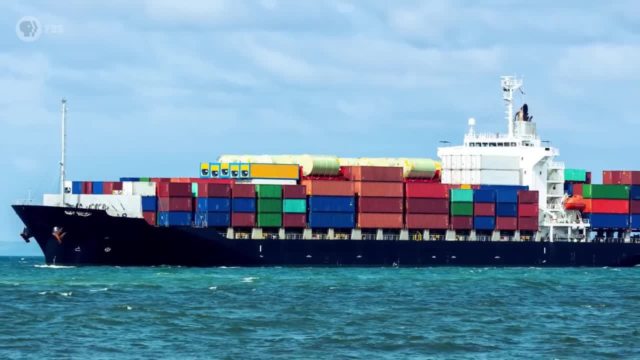 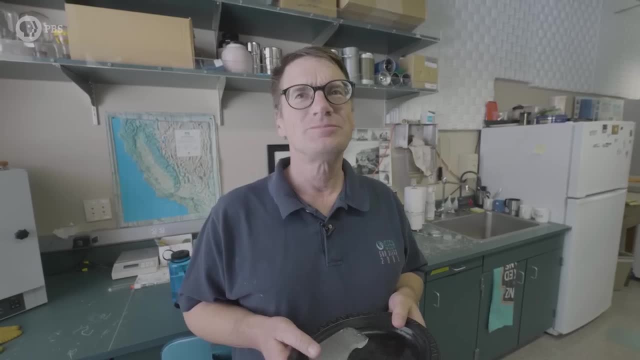 Once the core is pulled up, it's packed up and sent off, carrying a slice of history. It's a slow process, you know. it takes like a month for the ship to get here. Whether you're standing in the middle of the Amazon rainforest or at the North Pole, you're breathing roughly the same air. 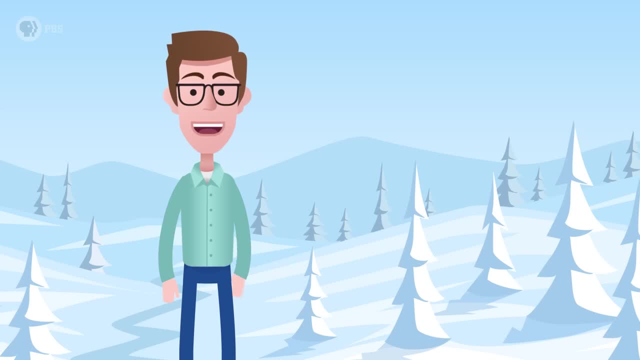 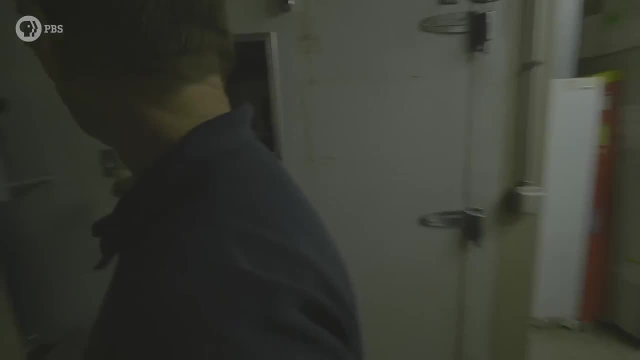 Our atmosphere is pretty much the same everywhere, which means that a tiny air bubble from that one spot is enough to paint a picture of what the entire planet's atmosphere looked like. This is the freezer, and we won't be in there long, so don't worry. 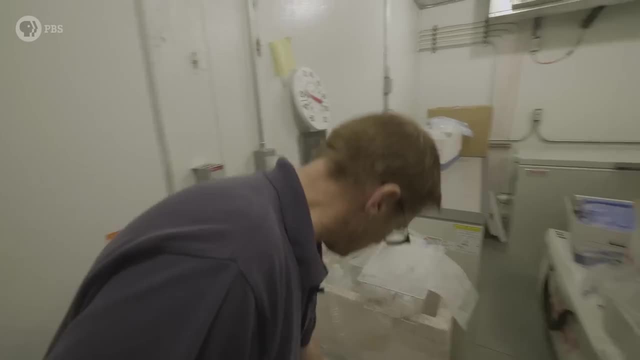 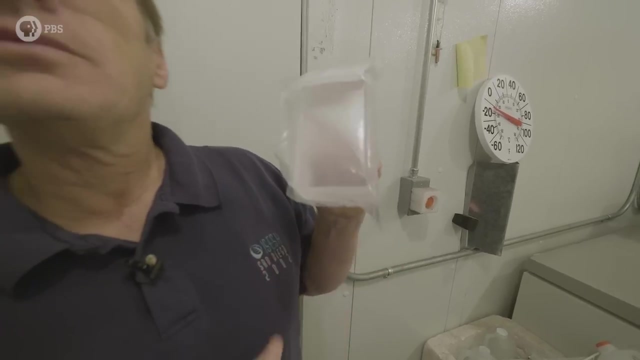 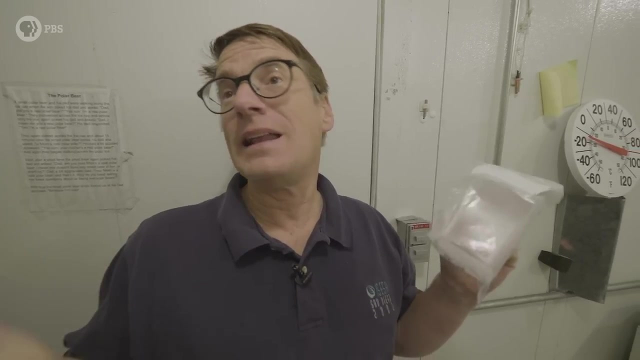 This is what a typical ice core sample actually looks like. Notice that there's no bubbles. That's because when you get below about 600-700 meters, the pressure is so high that the air turns into something called a clathrate, which is an ice-like substance. 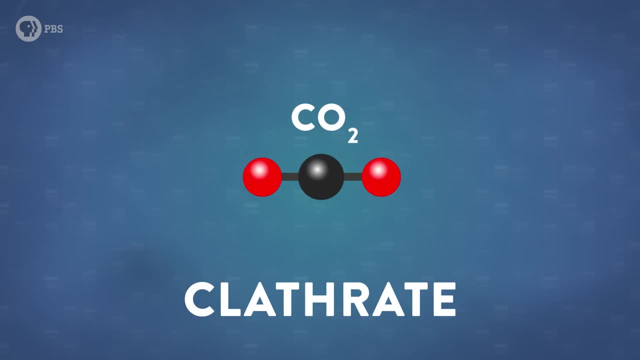 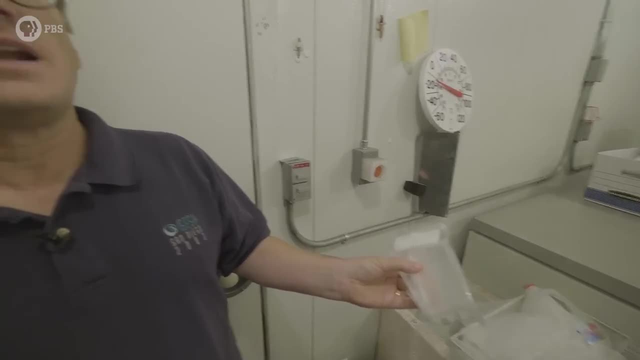 Clathrates are crystals where, instead of bubbles, the molecules are trapped in a cage made by the bonds between frozen water molecules. There's still gas in there, There's still gas molecules, But they're not in a gas phase Man. the patterns are so cool. 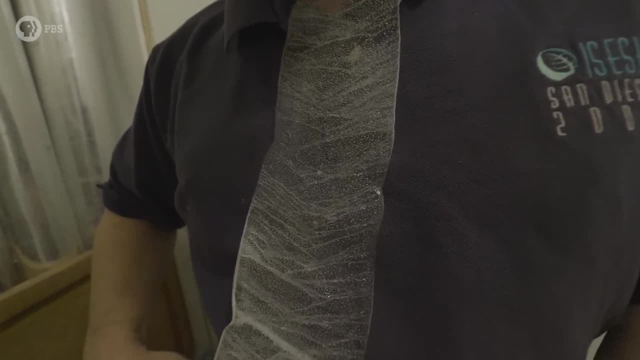 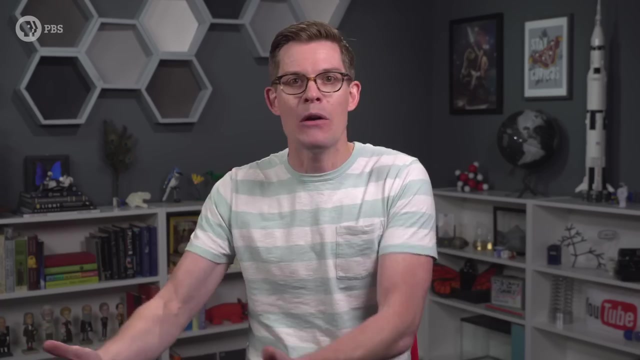 You must just see, like randomly, such cool ice phenomena. Oh yeah, It's cold in here, This cold. Funny how that works. yeah, Okay, but how do you get the ancient air out of the ice to measure it? 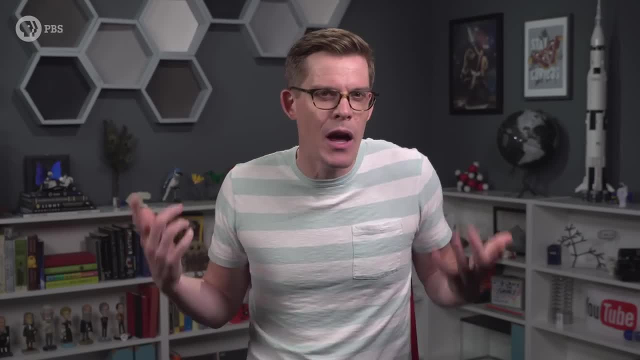 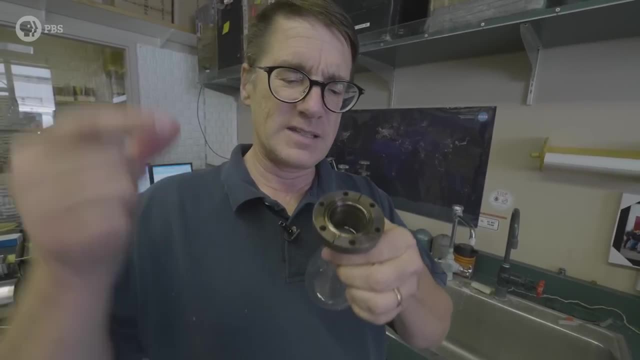 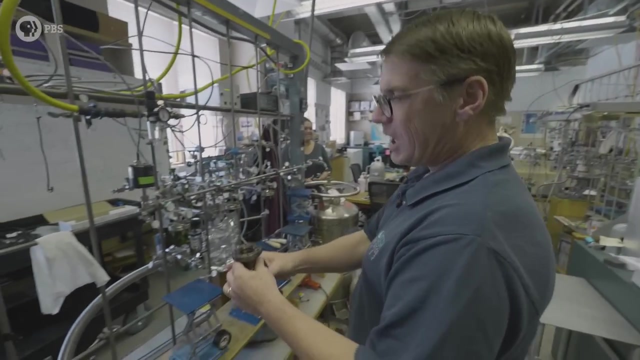 I mean without contaminating it with all this air around us. So this is how we actually extract the ancient air: if you will Take a piece of ice and put it in a vacuum flask like this And pump out all of the air, the modern air that you know, the air we're breathing right now- using a vacuum line. 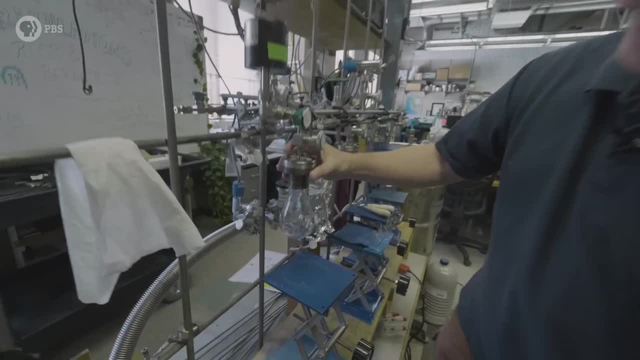 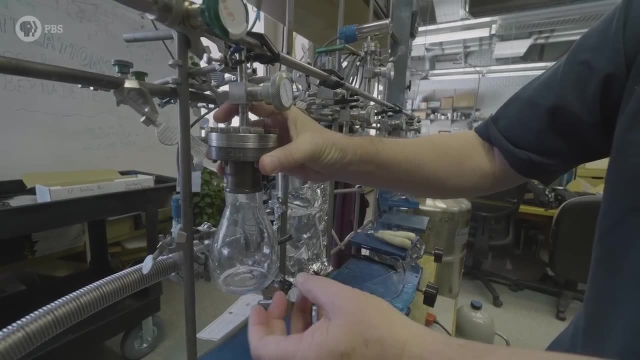 This is a vacuum pump here, So we make a seal and we pump out all the modern air And then we close this valve And then you only have an ice cube and a little bit of water vapor, but no air, And then you melt the ice. 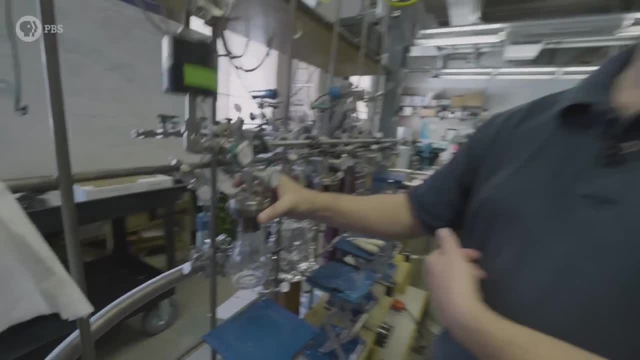 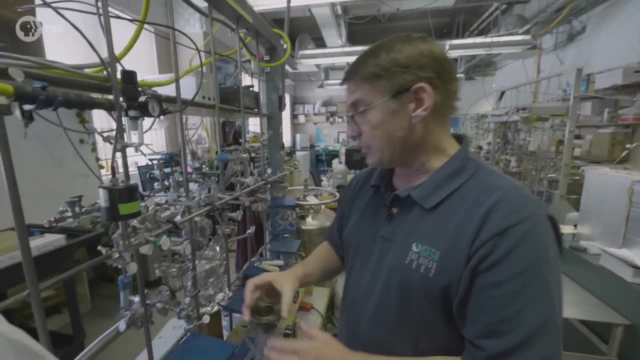 And the melting of the ice releases those little air bubbles. So because you got rid of all the now air, the only gases that are coming out are the ones that are trapped inside the ice Right, And so then, once we've done that, we can purify the gas a little bit by freezing the water. 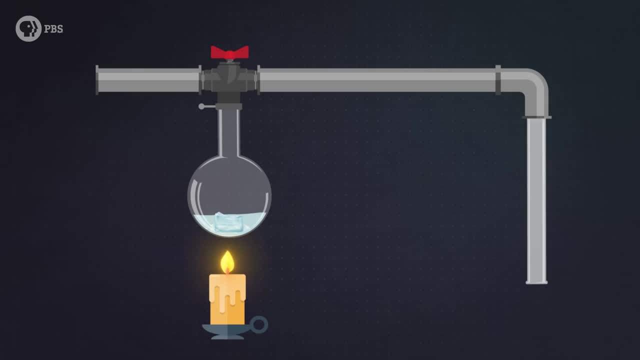 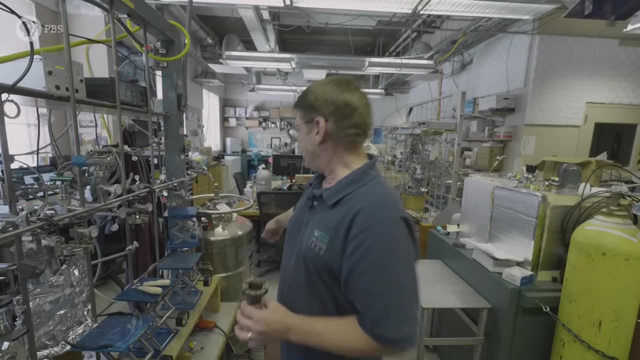 So they pump out all the modern air, melt the ice to let the ancient atmosphere vaporize, refreeze the water and pump that ancient atmosphere out so it can be measured. This is a liquid helium tank, so it's cold enough that it's at 4 Kelvin. 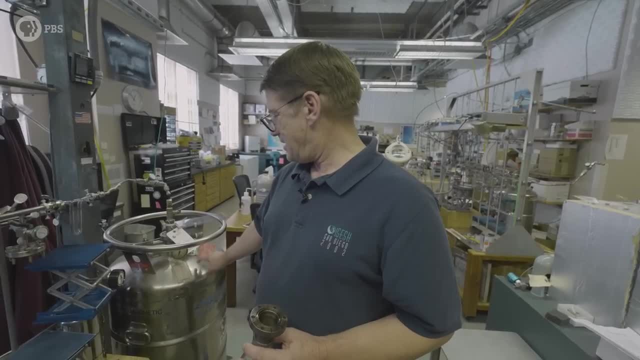 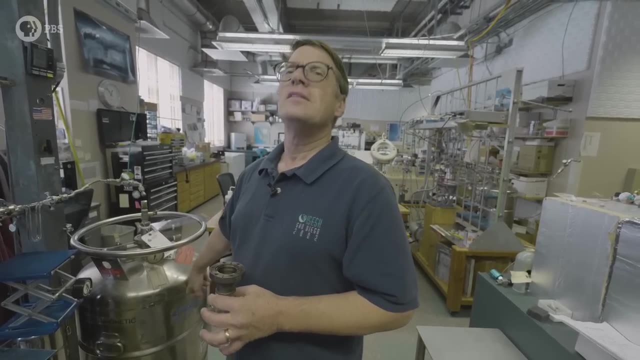 Okay, Wow, Four degrees above absolute zero. It's cold enough that all the air actually condenses and turns into ice, air ice, Every gas will. Every gas, except helium. Yeah, Then we take it over here, and this is the analysis part of it. 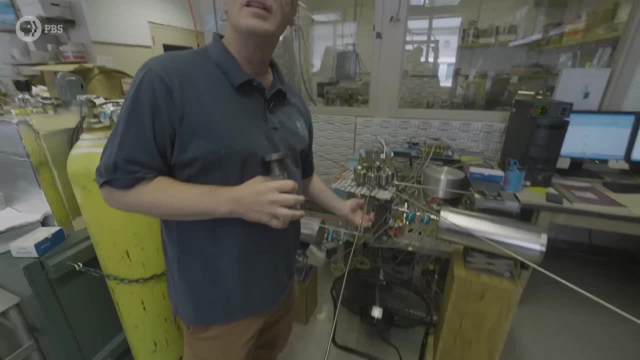 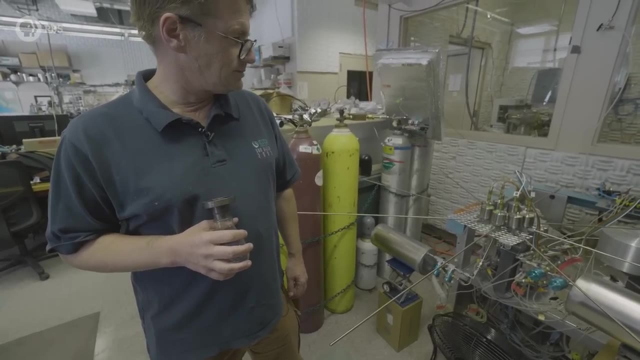 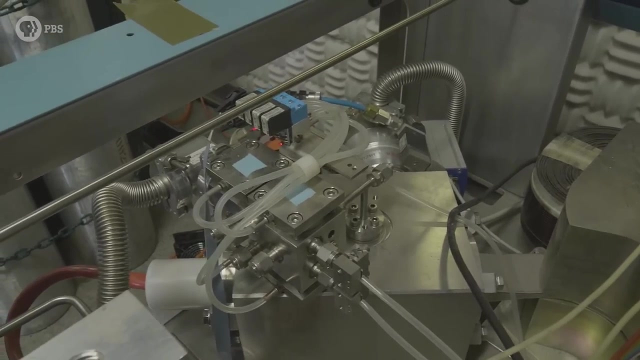 So this little tube is actually a bottle. It's a very long, skinny bottle that's capable of dipping itself into the liquid helium. You wouldn't want to be getting your own hands too close to 4 Kelvin. No, The frozen air gets put into this a mass spectrometer, which is a machine that we use to measure the masses of really tiny things. 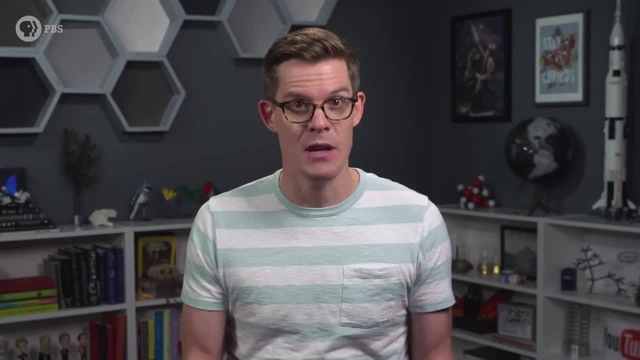 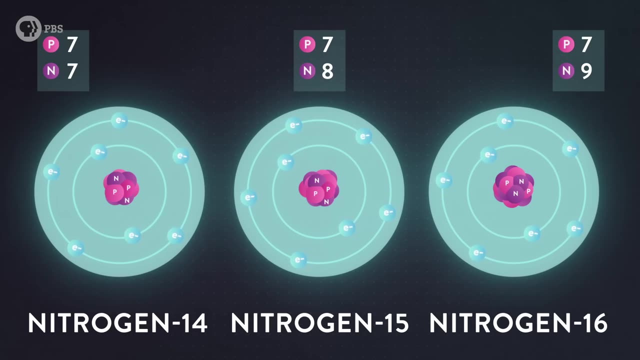 We measure the chemical composition of the atmosphere using isotopes. They're like different flavors of atomic elements. The isotopes, those flavors of elements, have unique masses, and the mixture of them in the air bubbles can tell us all kinds of things about ancient Earth. 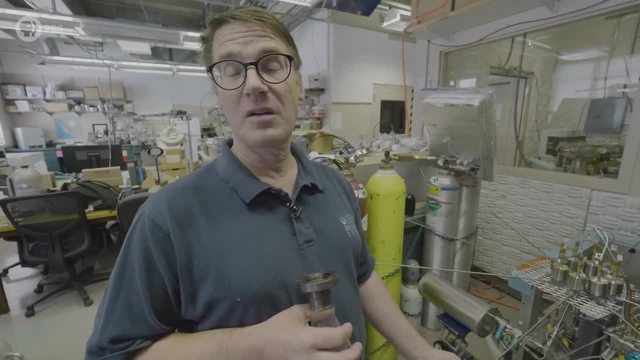 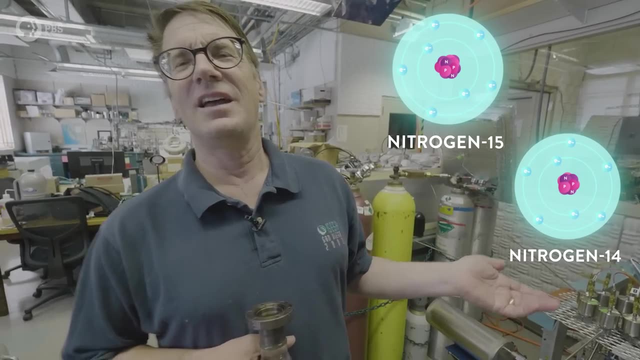 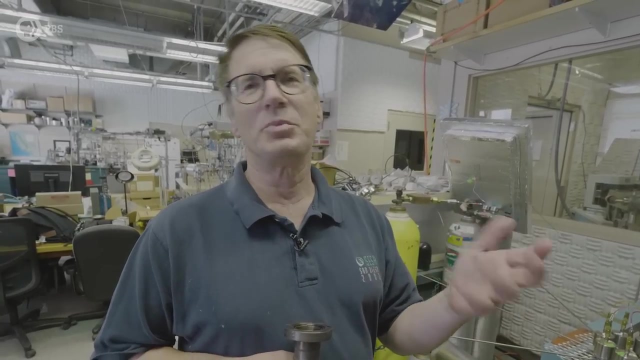 We use the isotopes of nitrogen to tell ancient temperature, basically at the time that the snow has fallen. Ordinary nitrogen has a mass of 14, and the rare isotope, nitrogen-15,, has a mass of 15.. So it turns out the relative proportions of N-15 and N-14 are sensitive to temperature. 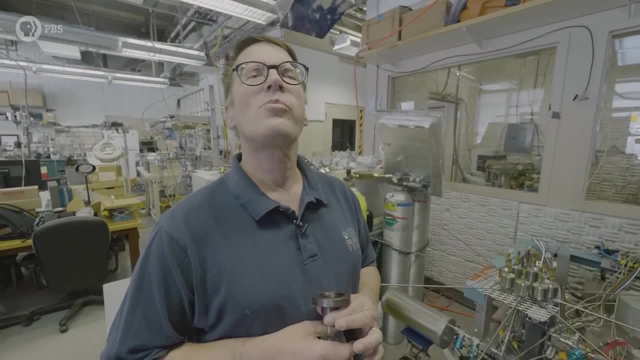 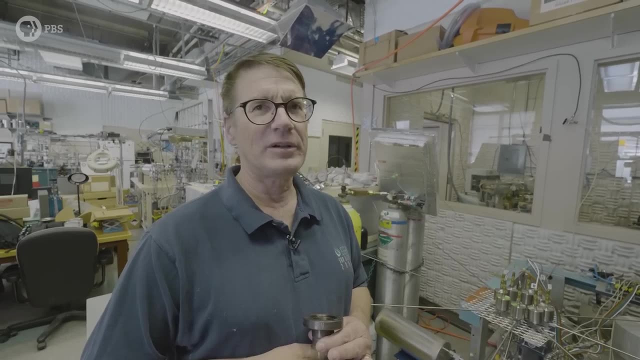 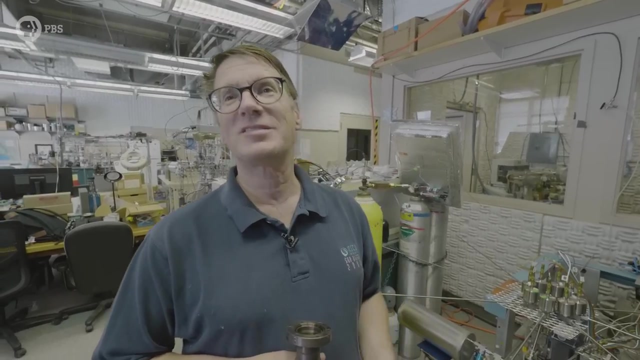 So whatever the temperature is at a particular time, it's creating different mixes of different flavors of gases in the atmosphere. That's right, Like a fingerprint for the temperature, Exactly yeah. And that's trapped in air bubbles for posterity. So the sample here starts out waiting its turn. 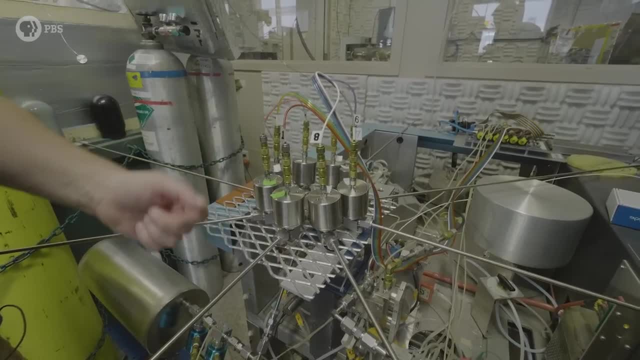 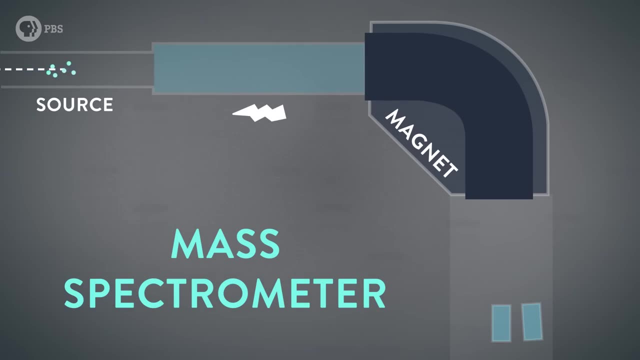 When its turn comes, this valve opens and then the sample goes through this little tiny tube and it leads very slowly into the actual mass spectrometer which is here. Then it gets accelerated by a 3,000 volt electrical gradient, makes the ions go really fast. 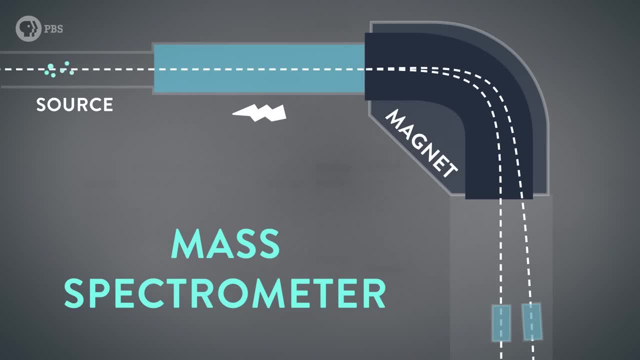 and then they hit this magnet And they're forced to make a 90 degree right turn And in doing so, heavy things like N-15 try to go straight and lighter things like N-14 get bent more. It's like being in a car. 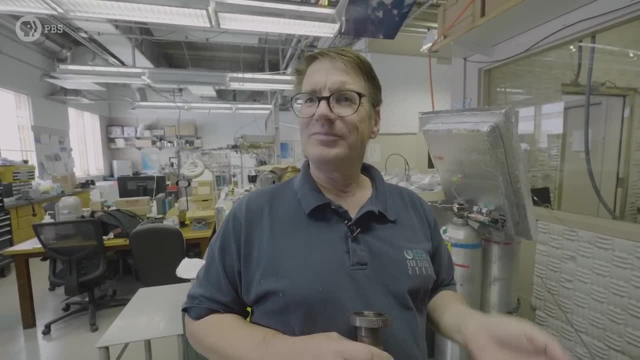 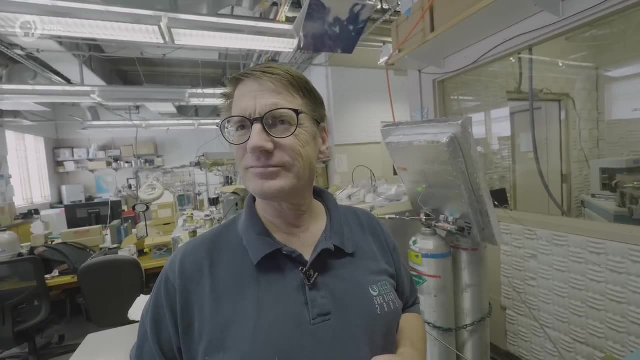 Exactly, yeah, So you can't turn as fast in a big heavy car, So they swing out and then the detector is seeing what's swung out farther. So you're getting resolution of things that differ by a single neutron when they're flying through that curve. 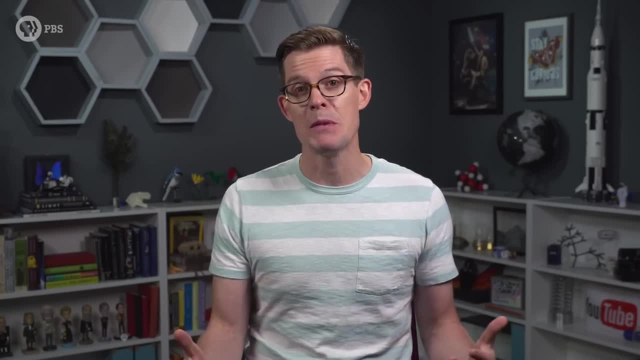 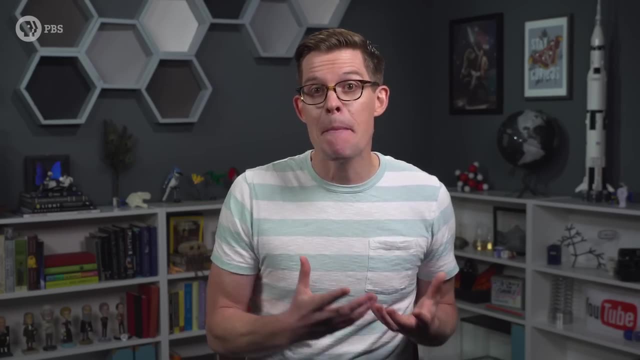 Yep, That's pretty cool. The same idea can be used to find out more than just temperature. Labs all over the world use elements trapped in air, trapped in ice cores, to paint a map from our distant past to today. Oxygen isotopes can tell us how oceans changed. 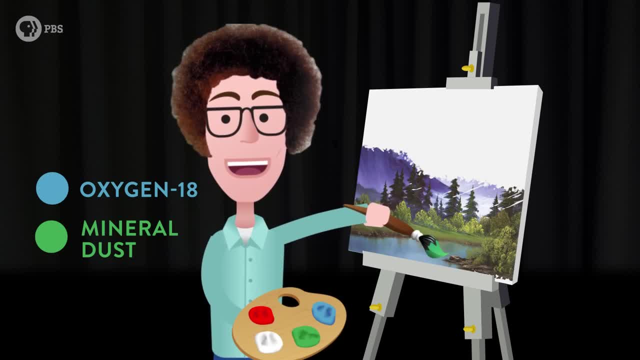 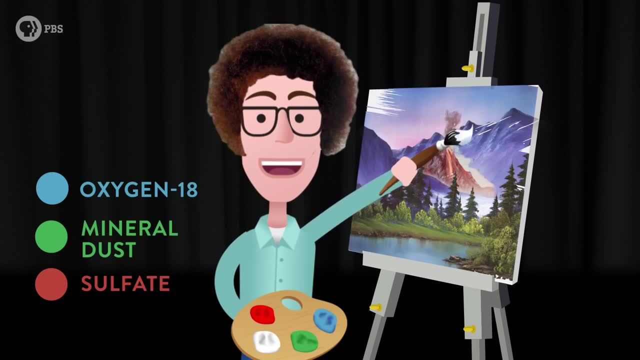 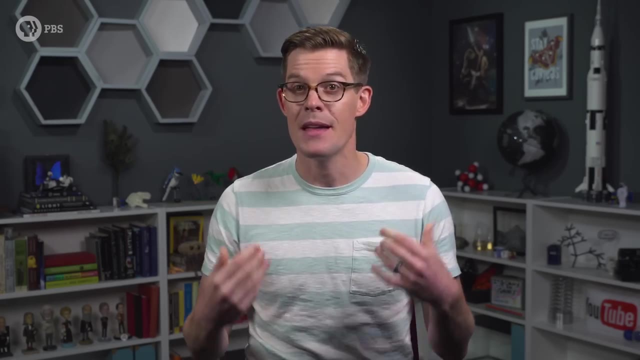 Mineral dust tells us about how the atmosphere moved around. There are chemical clues about early volcanoes, But maybe most importantly, we can trace changing levels of carbon dioxide. So the climate has changed before. How do we know that this time it's us? 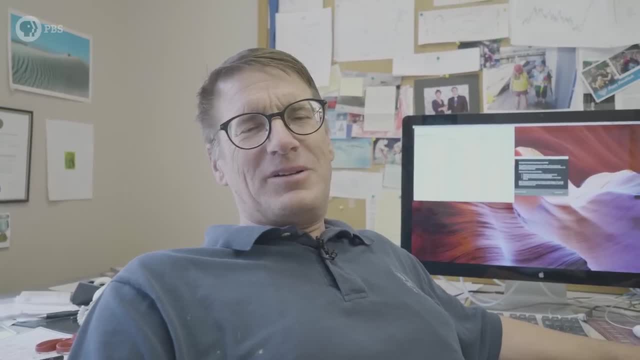 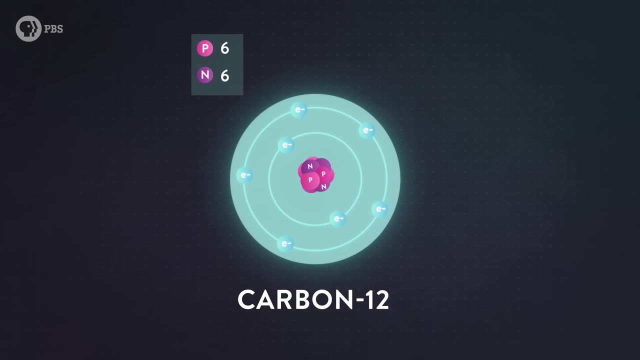 So the way we know is that, just like we talked about for nitrogen, it turns out that carbon and carbon dioxide also has two flavors: Carbon-12,, which is ordinary carbon, and then a very rare form of carbon, carbon-13.. That's how we know that it's human-caused. 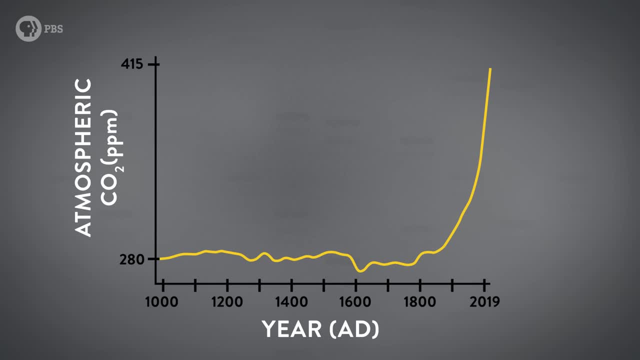 The atmosphere as it goes up in concentration, CO2 concentration, the carbon-13 is taking a nosedive, And that's not what would happen. What would happen if it was natural CO2?? Because fossil fuel CO2 is very depleted in carbon-13. This comes from the fact that plants prefer to eat CO2 made of carbon-12.. And when we burn fossil fuels made from those ancient plants, the fraction of carbon-12 in the atmosphere goes up, while carbon-13 goes down. We've only been measuring carbon dioxide in the atmosphere since 1957.. 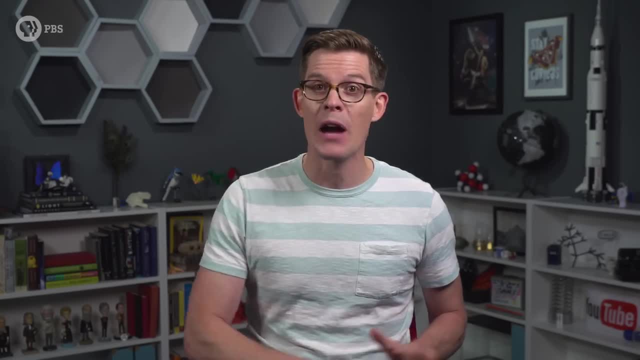 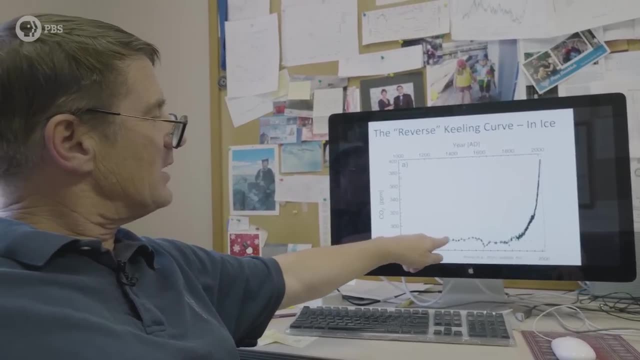 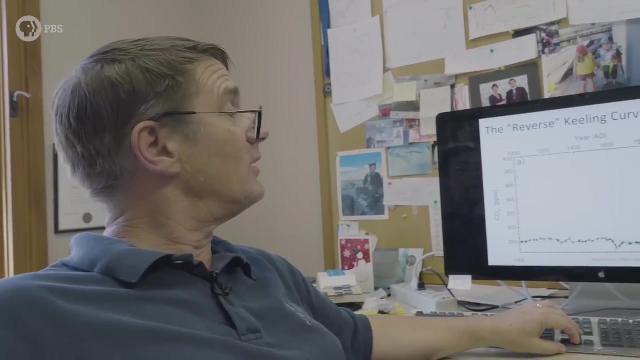 But using the data from ice cores we can trace levels back way way farther. And this is what we see. CO2 was pretty flat for most of the past thousand years: all around 280 parts per million. Now we're going to add in the carbon-13 abundance record. 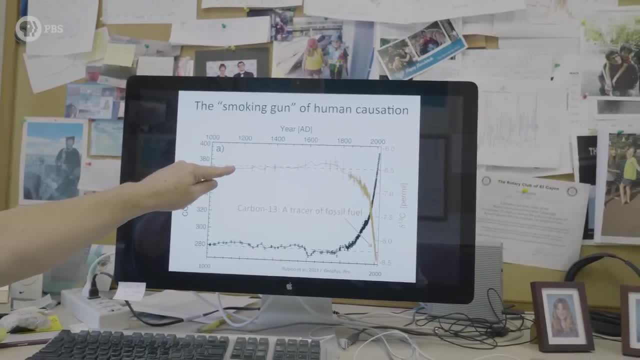 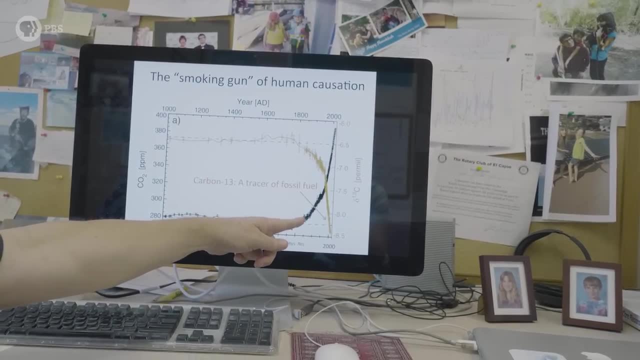 That's this gold line here. You can see that that was also pretty constant for most of the last thousand years. But then around 1850, right when the carbon dioxide concentration started to rise- the carbon-13 abundance started taking a nosedive. 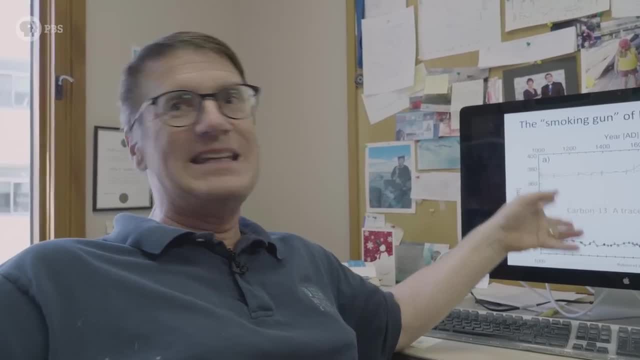 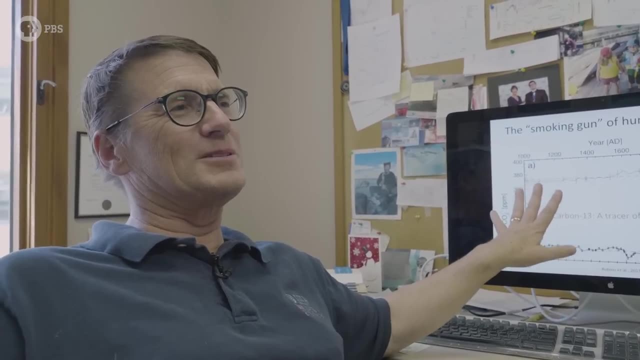 So this really unambiguously tells you that humans did it. That's why I call it the smoking gun of human causation. There's lots of other ways we know, but this is the simplest to explain. We are moving into uncharted territory. 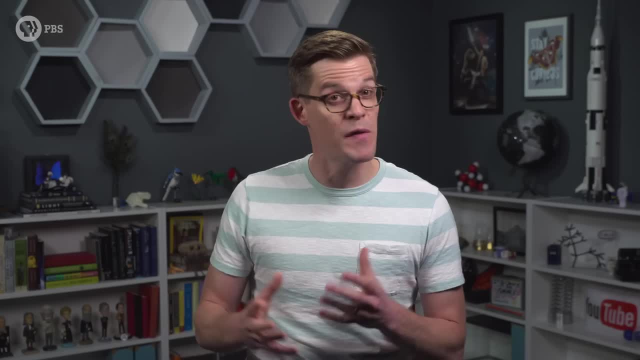 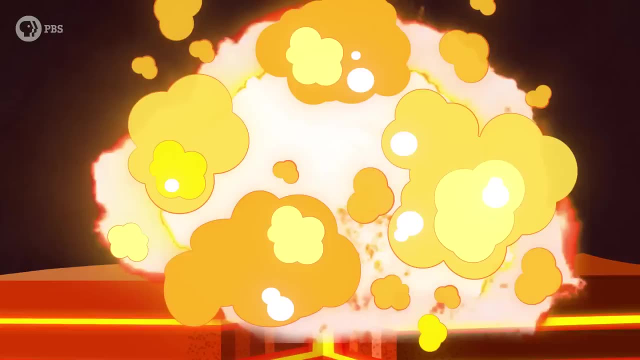 I mean, the last time something like this shows up in the ice record is around 55 million years ago, when a volcano popped up under an oil field and cooked basically everything. It sent all of the carbon dioxide into the atmosphere. So the carbon dioxide. 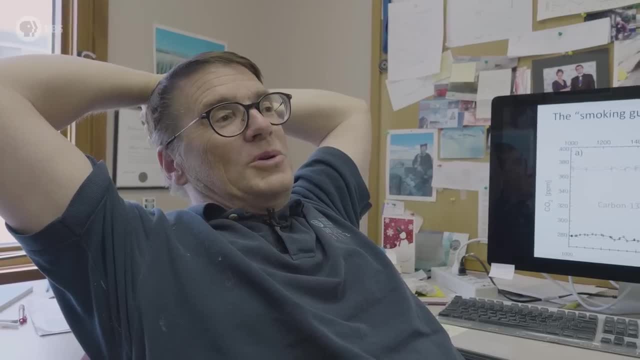 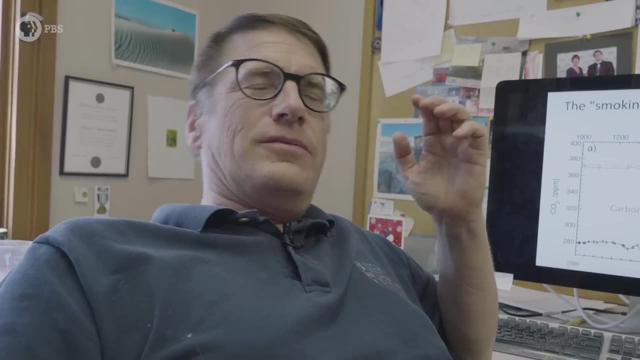 in the atmosphere shot up. We think it basically quadrupled And the climate warmed by six degrees. The most important thing is, just right away, to solve this global warming problem. We don't have much time left. We've got to put aside all of our political differences. 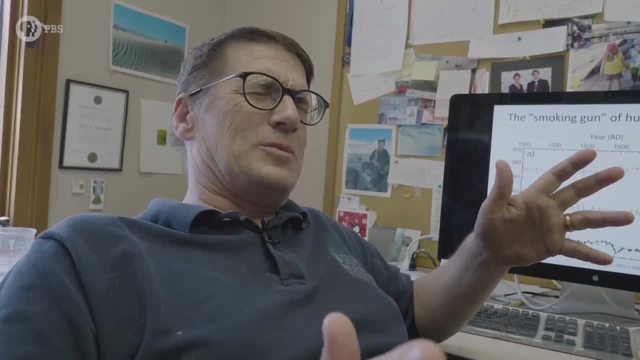 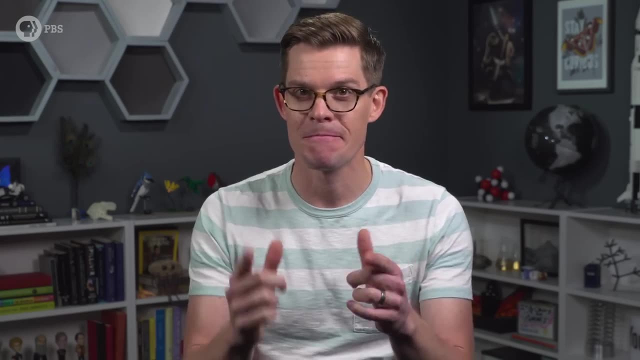 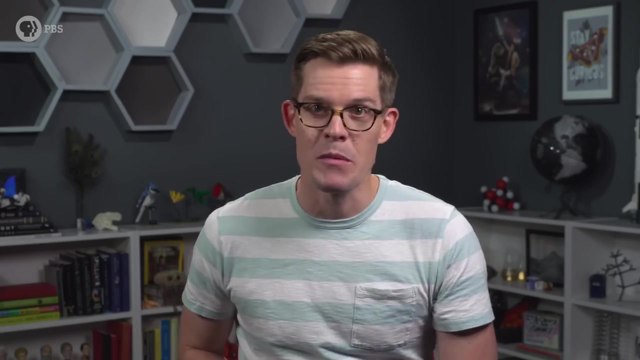 The health and well-being of the planet is so much more important than anything else. And we can do this. I know we can. We can, but will we? I hope so. Stay curious. Hey, thank you for sticking around, because PBS Digital Studios wants to hear from you. 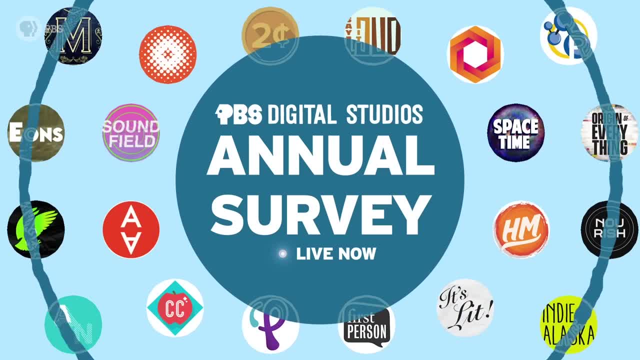 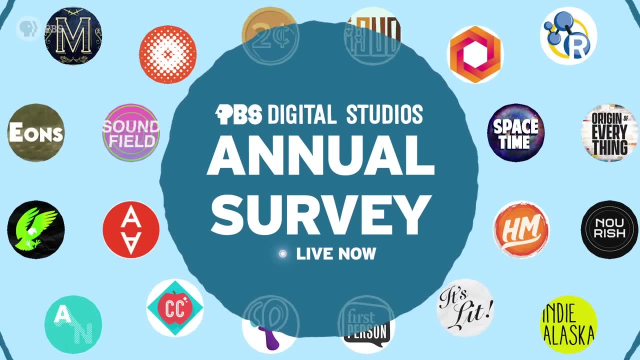 We do a survey every year that asks about what you're into, what your favorite PBS shows are and things that you'd like to see more of from PBS Digital Studios. You even get to vote on potential new shows. All of this helps us make more of the stuff that you want to see. 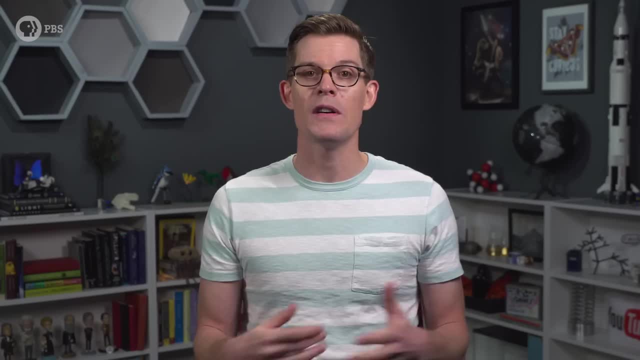 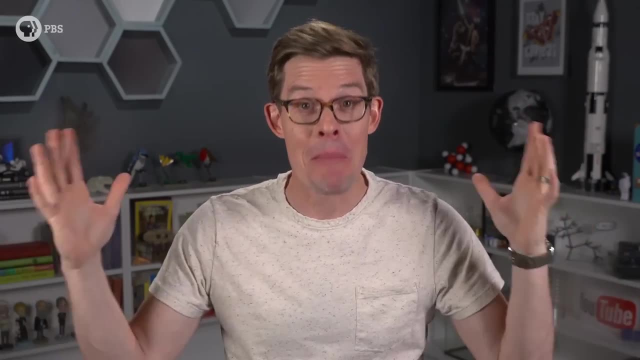 The survey takes just about 10 minutes and you might want a sweet T-shirt if you fill it out. There's a link down in the description. Thank you so much. We'll see you next time. It's Okay To Be Smart is now on Patreon.